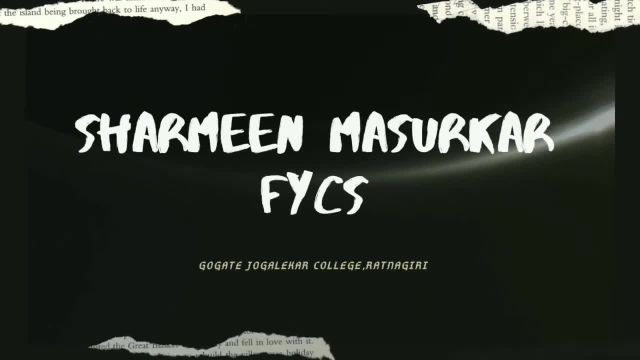 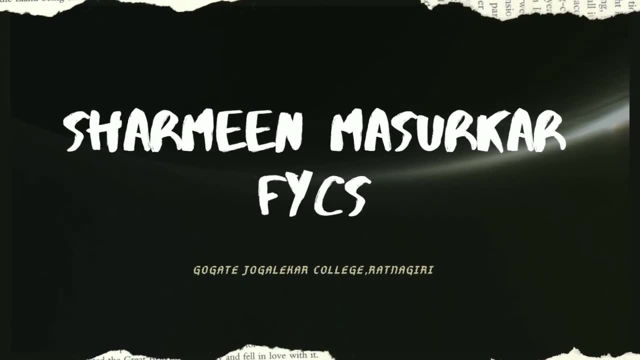 My name is Sharmeen Masurkar. I am a student of FYBSC Computer Science in Guptek Zoghalekar College, Ratnagiri. Today in this video, we are going to discuss how we solve a recurrence relation using backtracking method. 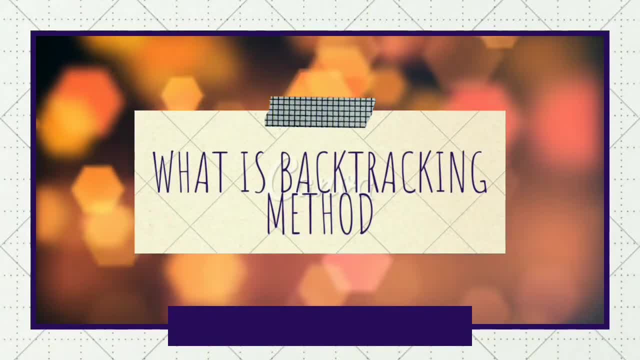 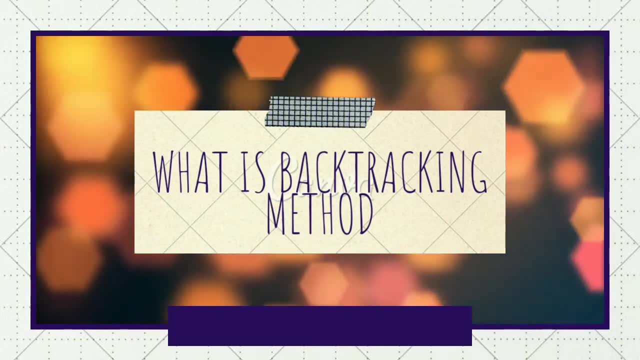 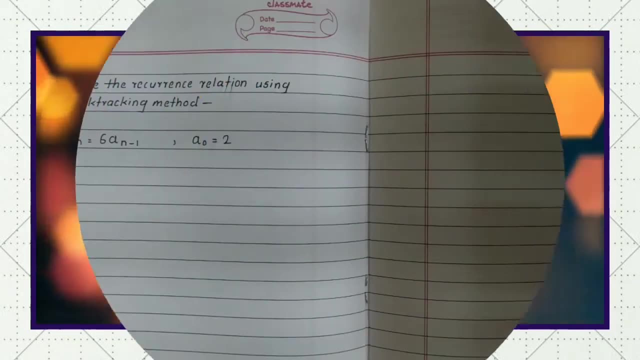 Now, what is backtracking method? It is an algorithmic technique for solving problems recursively, by trying to build a solution incrementally And removing those solutions that fail to satisfy the constraints. Let's move on to the problem. We have to solve this recurrence relation using backtracking method. 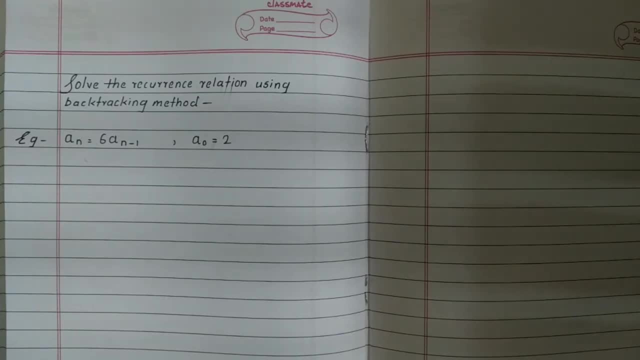 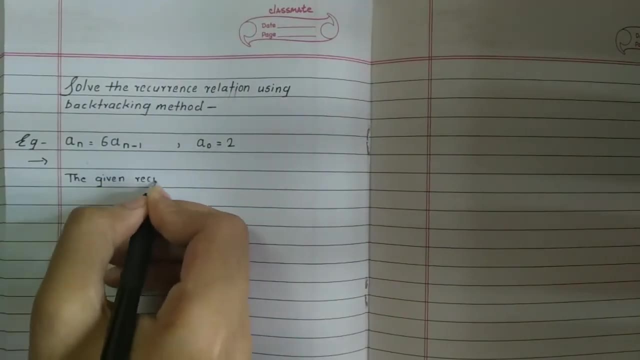 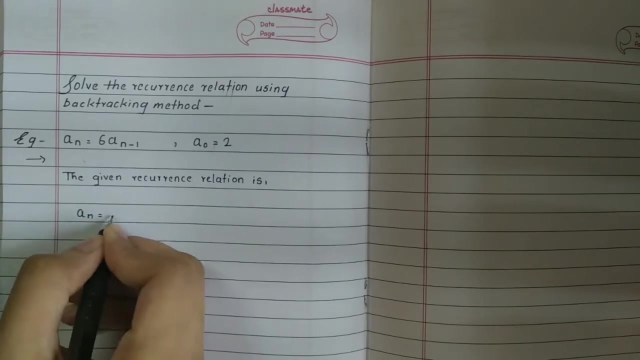 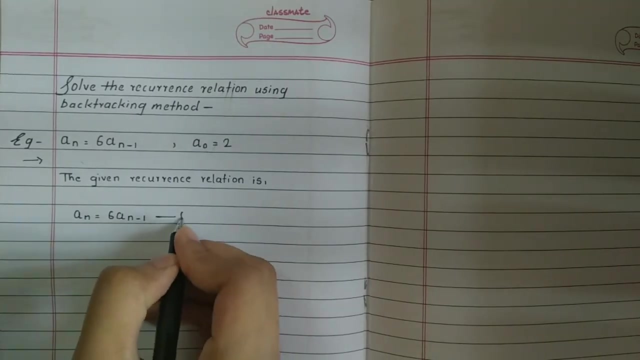 And the example is an equals to 6an-1 and the value of a0 is 2.. Let's start the solution. The given recurrence relation is an equals to 6an-1. We'll give it as equation number 1.. 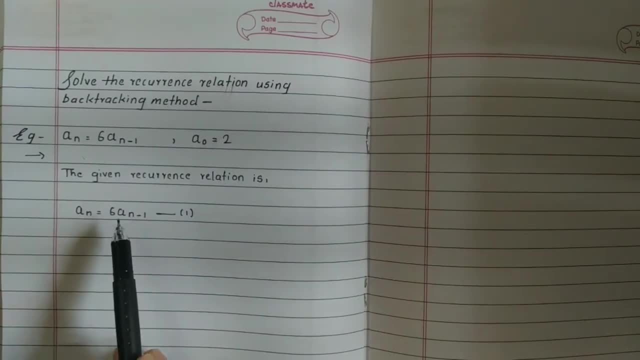 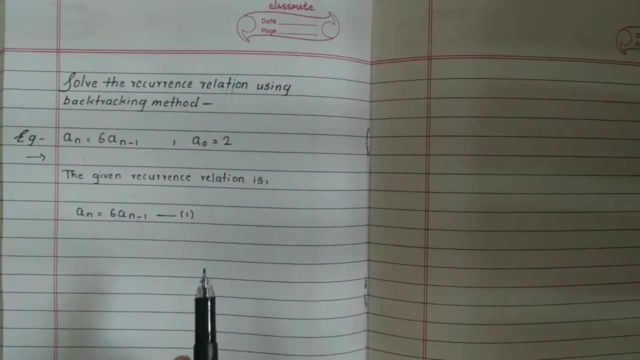 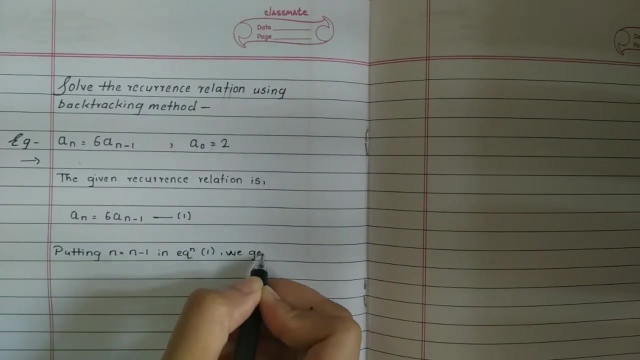 Now over here, we have to find the value of an-1.. And to find the value of an-1, we have to put n equals to n-1 in equation number 1.. So by putting n-1- n equals to n-1- in equation number 1, we get. 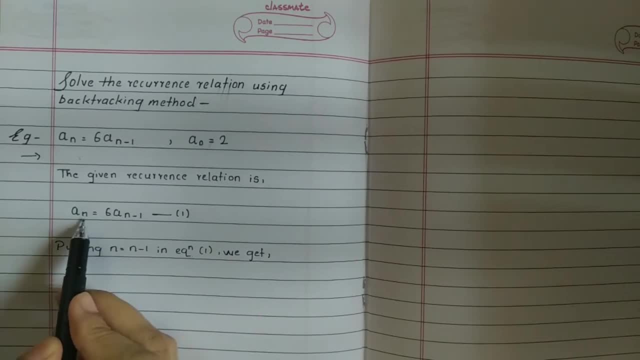 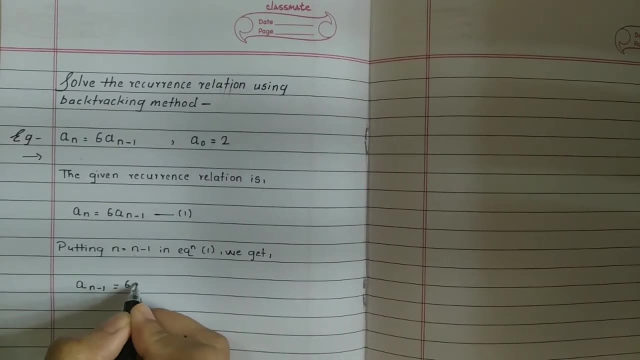 a. at the place of n, we'll write n-1.. That is n-1 is equals to 6a. at the place of n, we'll write n-1.. That is: n-1 minus 1 will remain as it is. 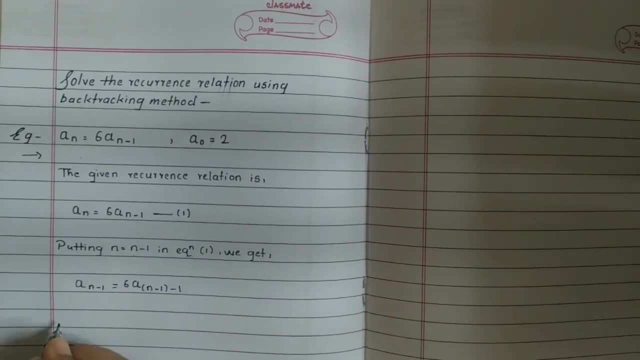 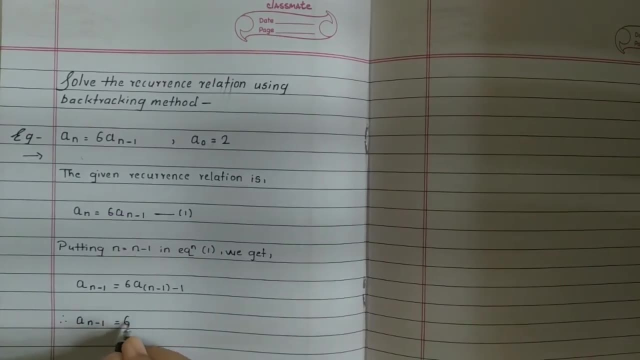 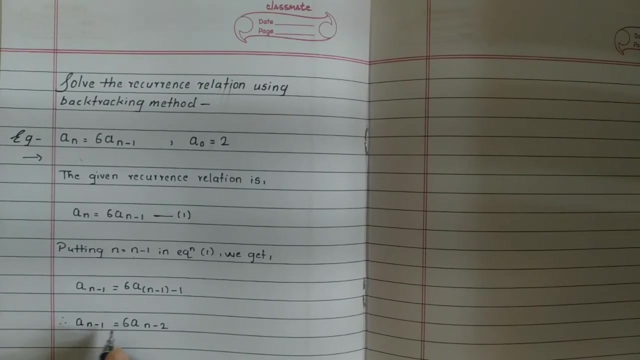 minus 1, and minus 1 is equals to minus 1.. Therefore we get the equation: an-1 is equals to 6an-2.. Here we got the value of an-1, that is 6an-2.. 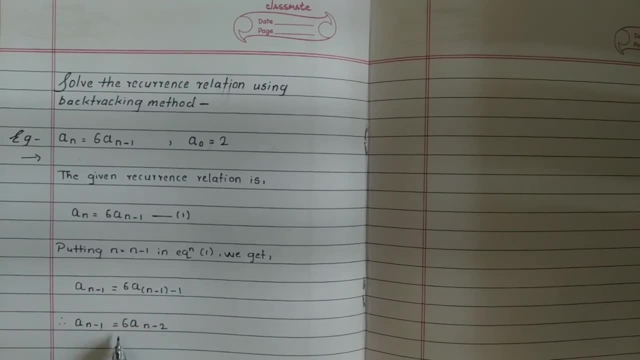 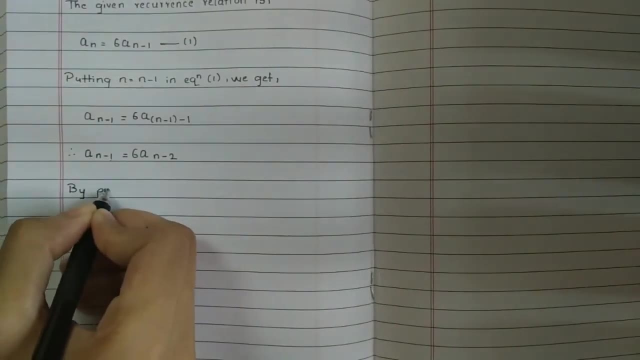 We have to put this value of an-1 in equation number 1.. Therefore, by putting the value of an-1, we get 6an-2.. Therefore, by putting the value of an-1, we get 6an-2.. 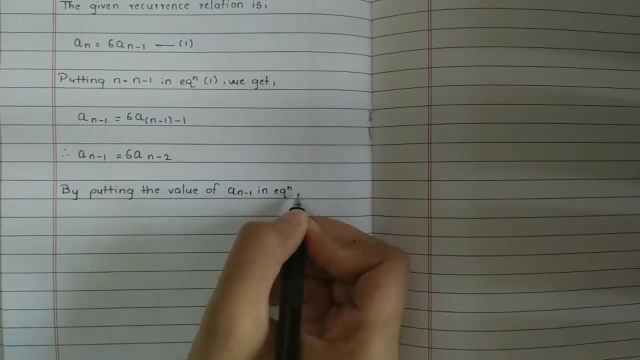 Therefore, by putting the value of an-1,, we get 6an-2.. and in equation number 1,, we will get 6an-2 at the place of an-1. in equation number 1, we get 6an-2,. that is our second prime value. 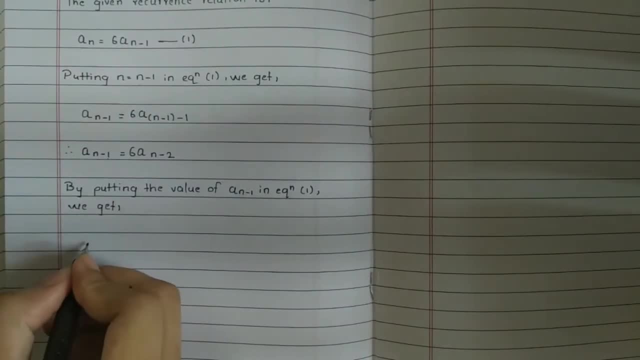 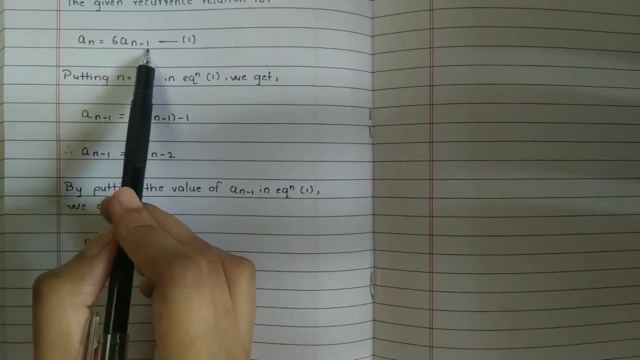 an is equals to 6 will remain as it is, and in equation number 1, we get 6an-2 at the place of an-1, we will get 6an-2, a-n it is: a-n is equals to 6. 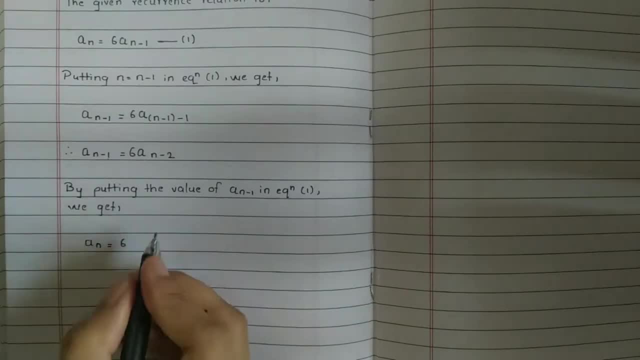 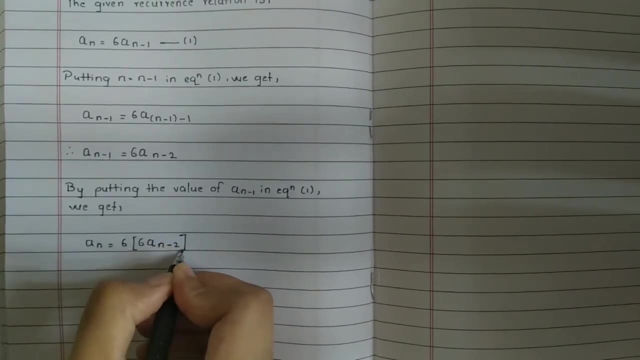 tf, as it is the value of the. at the place of an-1 we will write 6a-2ugh-n- Tf, as it is 6an-2.. Therefore we have n-1, and that is n-2.. 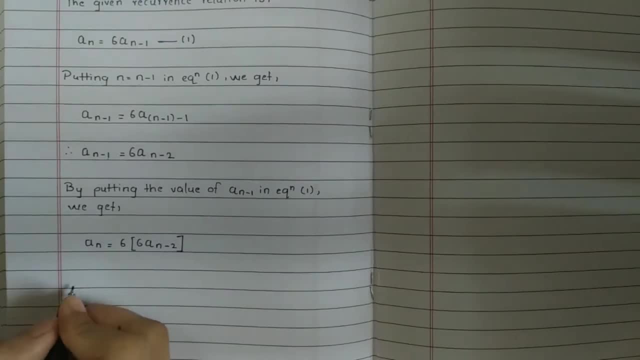 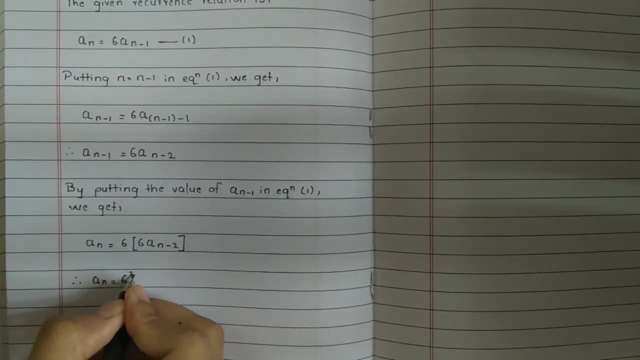 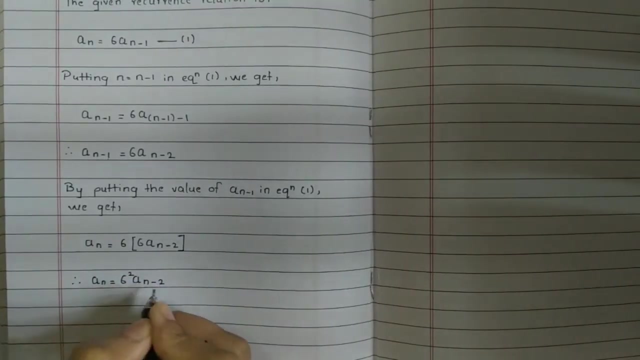 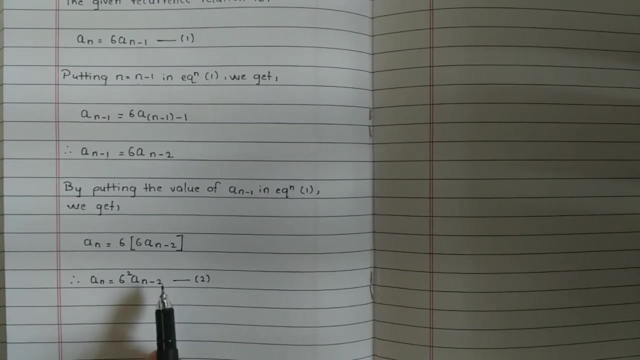 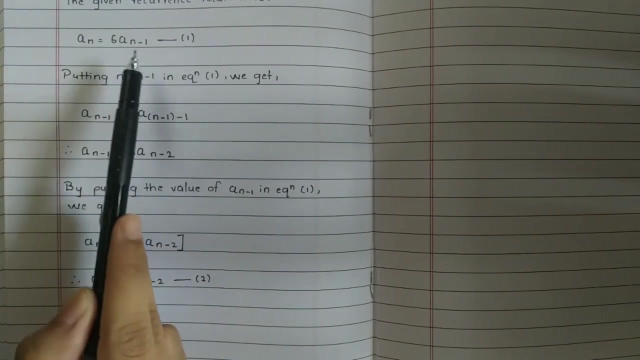 6x6 is equal to 6 square. Therefore we get the equation: AN equals to 6 square. AN-2 will remain as it is. We will give it as equation number 2.. Now again we have to find the value of AN-2.. Therefore we will put N equals to N-2 in equation number 1 rather than in equation number 2.. 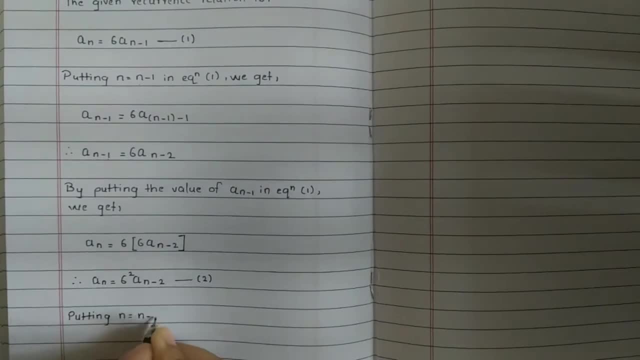 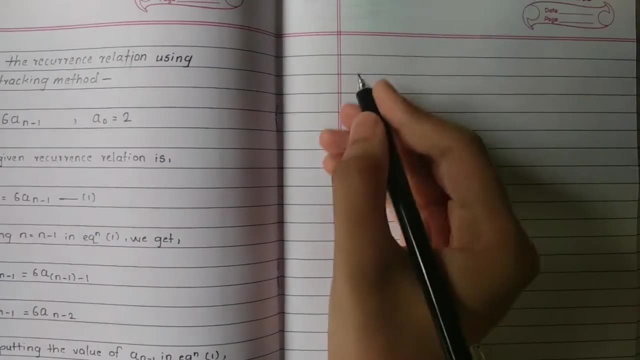 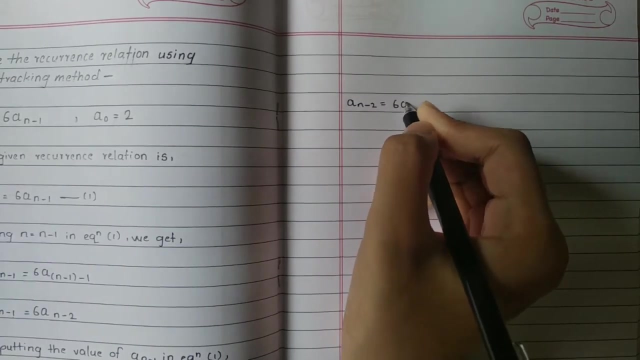 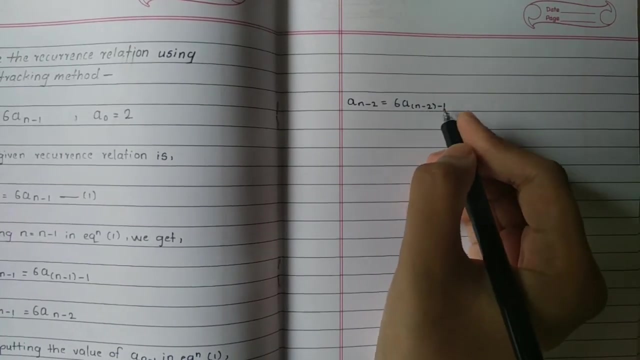 So putting N equals to N-2 in equation number 1, we get What we will get is AN-2 is equal to 6AN-2 and the remaining minus 1 will be as it is: Minus 2 and minus 1 is equal to minus 3.. 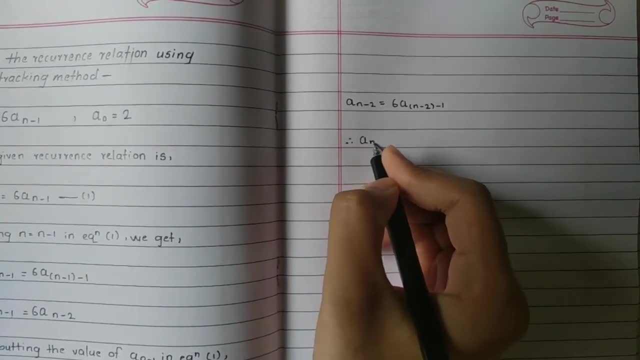 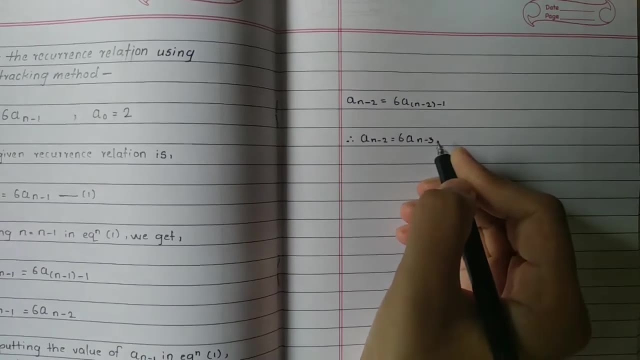 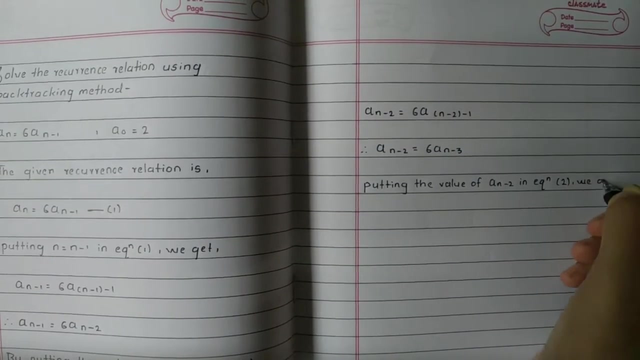 Therefore, the equation will be: AN-2 is equal to 6AN-3.. Therefore, putting the value of AN-2 in equation number 2, we get At the place of AN-2, we will write 6AN-3.. 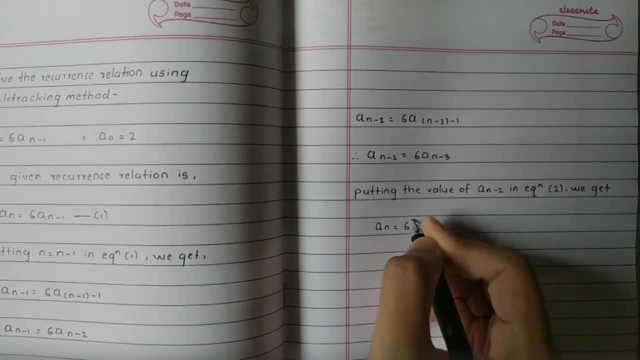 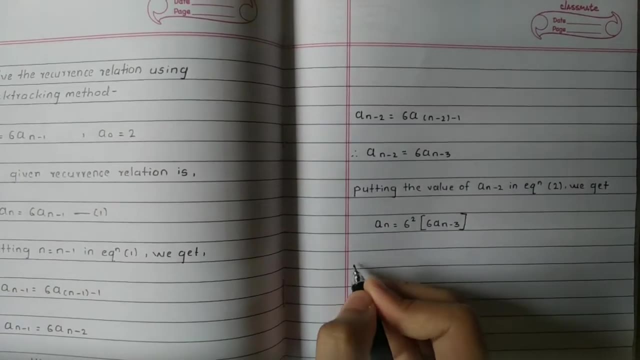 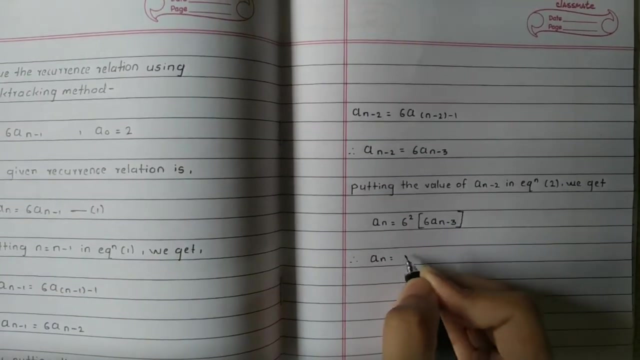 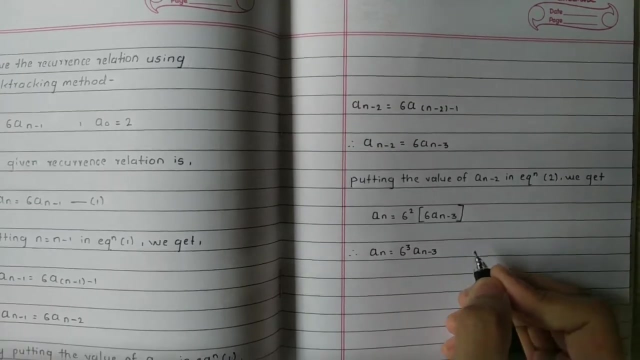 That is AN equals to 6 square into 6AN-3.. Therefore, 6 square into 6 will be equal to 6 cube. That is, AN equals to 6 cube- AN-3.. We will give it as equation number 3.. 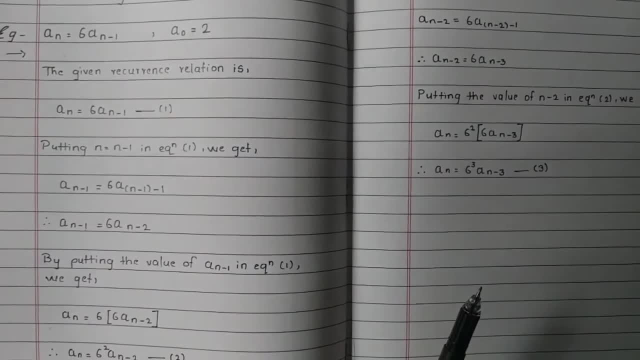 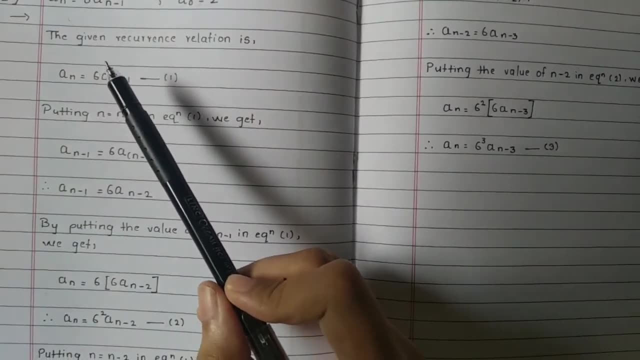 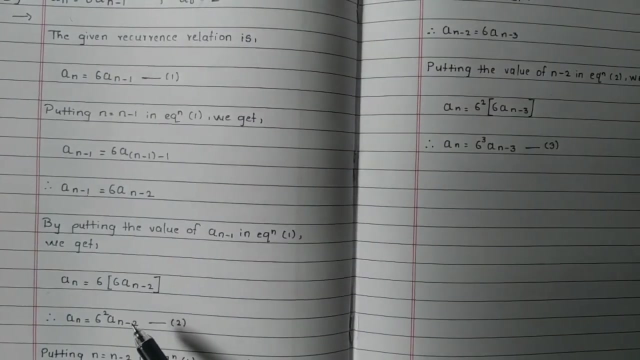 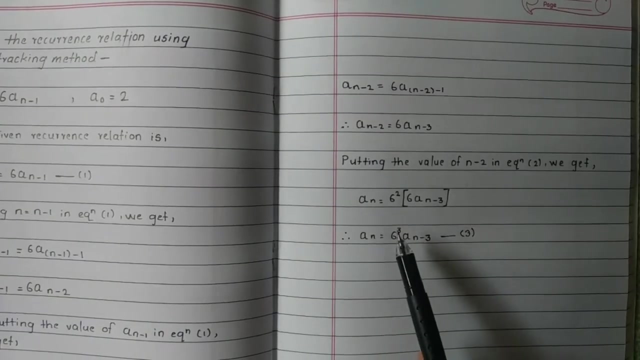 We have got three equations Now we can observe that whatever value is in the power of 6 is same over here, Like 1, 1,, 2,, 2,, 3 and 3.. As we move further, these numbers will frequently change. 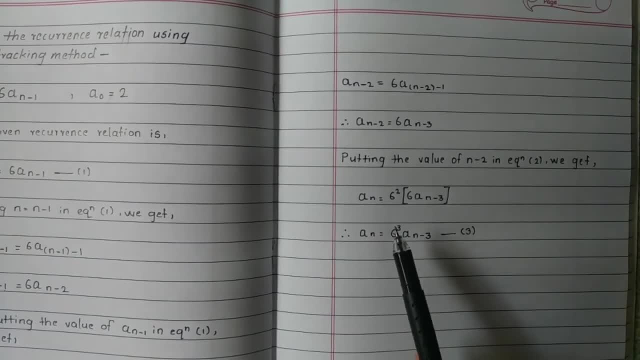 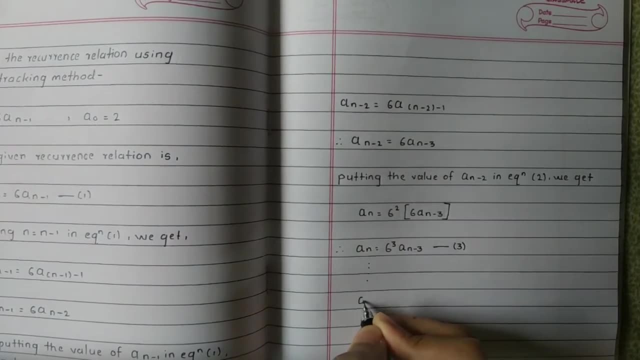 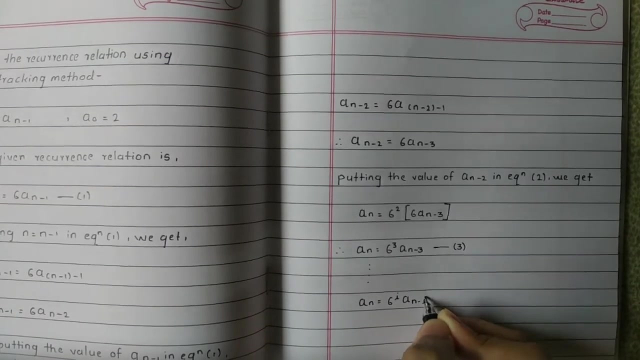 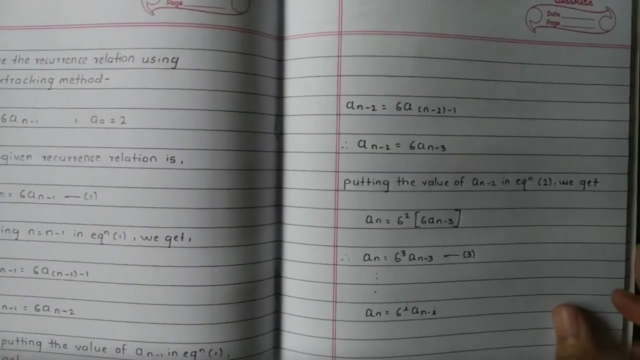 So we can write I at the place of 3.. Therefore we will get the new equation That is: AN is equal to 6 raised to I, AN-I Over. here we have given the value of A0. That is 2.. 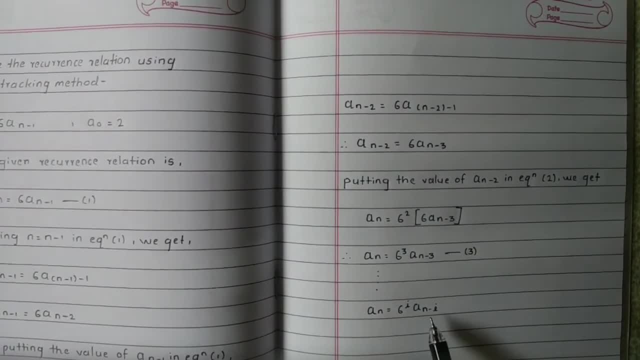 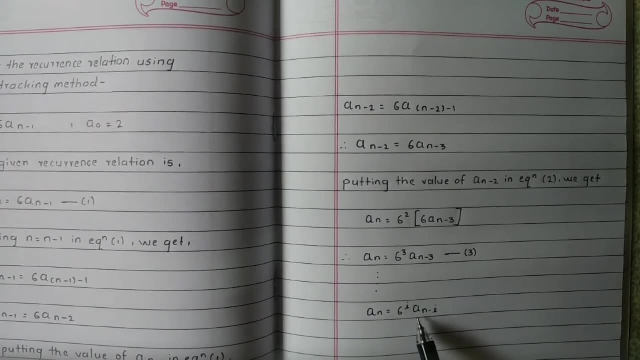 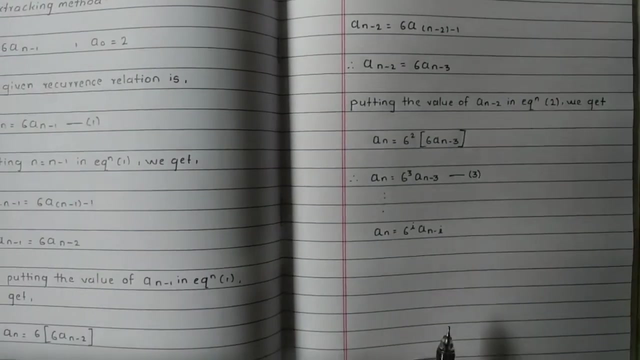 Now we have to make an arrangement in such a manner that we get A0 instead of AN-I. If we put I equals to N, then we will get A0.. As N-N is equal to 0. Therefore, putting I is equal to N, we will get. 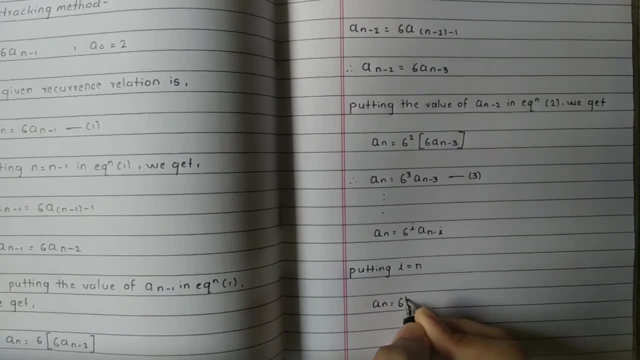 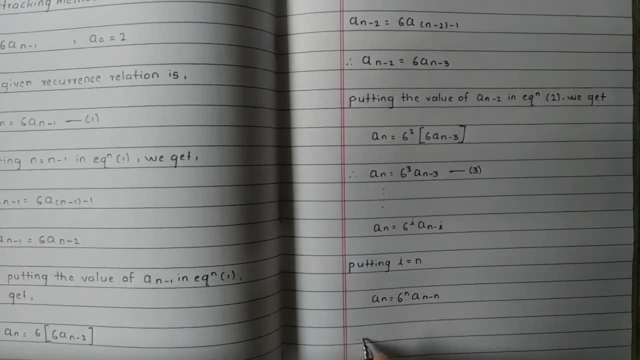 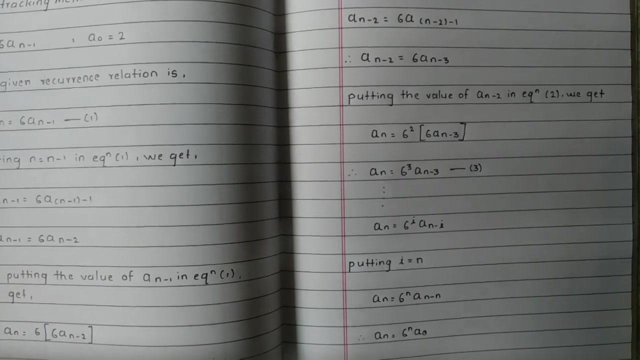 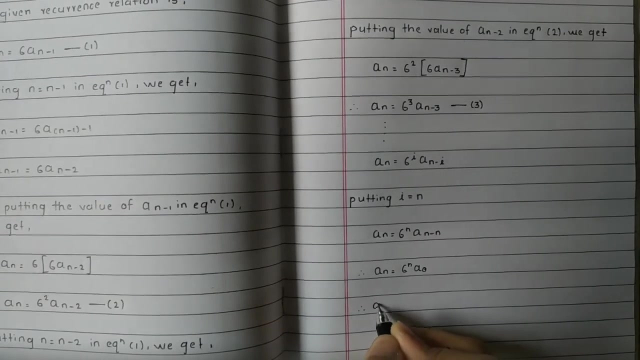 AN is equal to 6 raised to N- AN-N. Therefore, we will get: AN is equal to 6 raised to N- A0.. And the value of A0 is 2.. Therefore, we will get AN is equal to 6 raised to N into 2.. 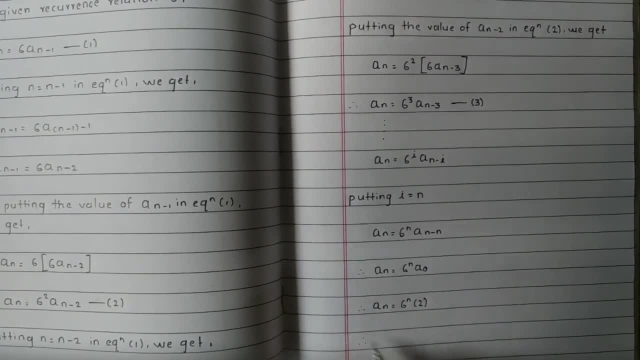 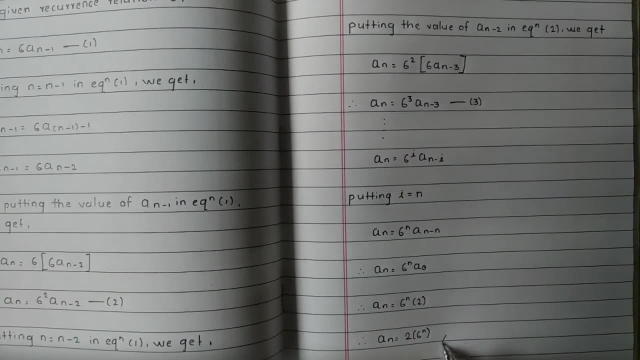 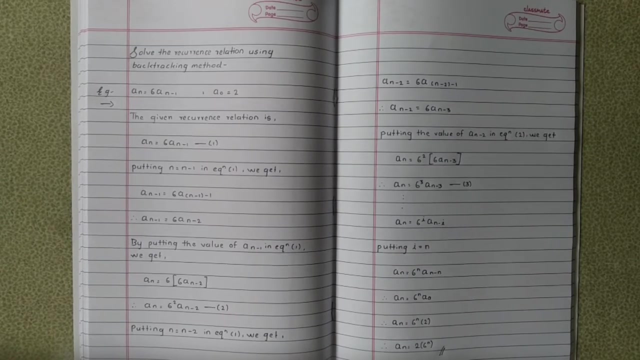 We have to arrange this equation. Therefore, AN is equal to 2 into 6, raised to N. This is the final equation we have got. This is how we solve a recurrence relation using backtracking method. Please do share and subscribe our channel.